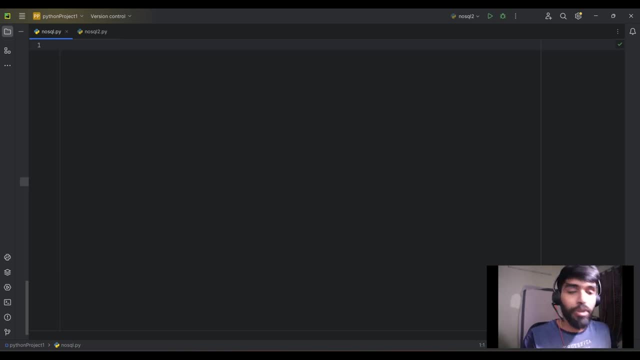 you Okay. so let's just start with my first code. So I'm just going to create a class, simple NoSQL TB. I'm just giving a name for my class And then I'm going to create a method. It's like a. 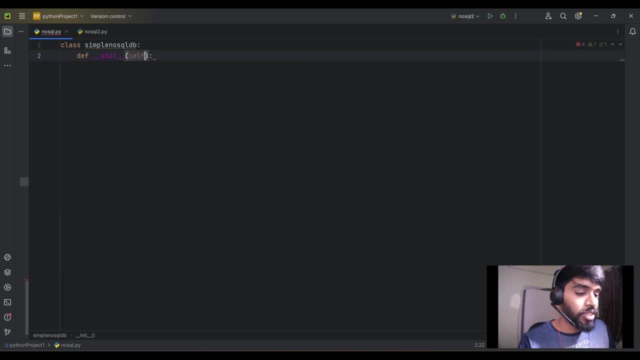 constructor And I'm just initializing the class with a self keyword And then self dot. I'm creating an instance variable for the particular initialization, So it could be any name. So here, in this case, I'm giving us a data, it could be any name. And here I'm giving a dictionary. it's an empty dictionary, I'll tell. 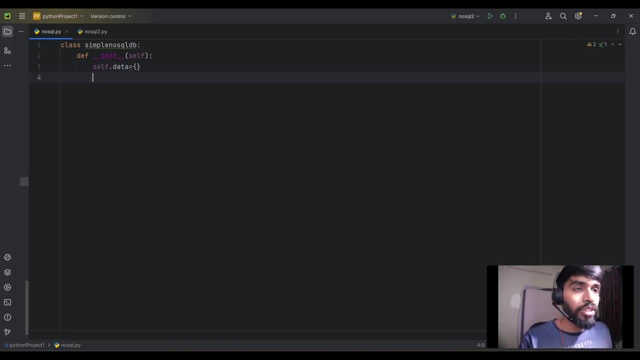 you the reason why I'm going with the empty dictionary. Okay, so now the agenda. I'm just have to create some functionality, like you have to do insert and then you have to do get, which is like select and get the output and delete and display. So this four functionality. 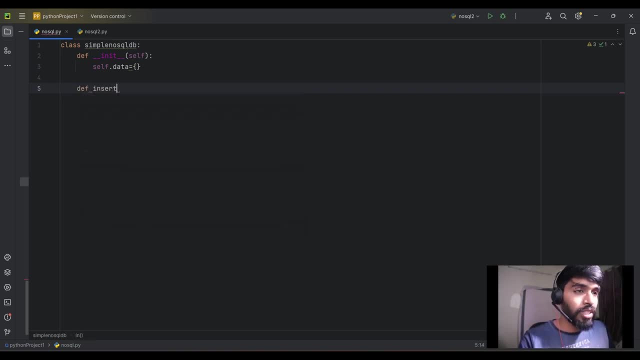 I have to implement. So let me start with insert. Okay so, and then I'll call self, because I have initialized with this class, So as a constructor, so I have to pass the self as a first parameter. And then I'm giving two variables as key and value. Okay so, totally, I'm having like three. 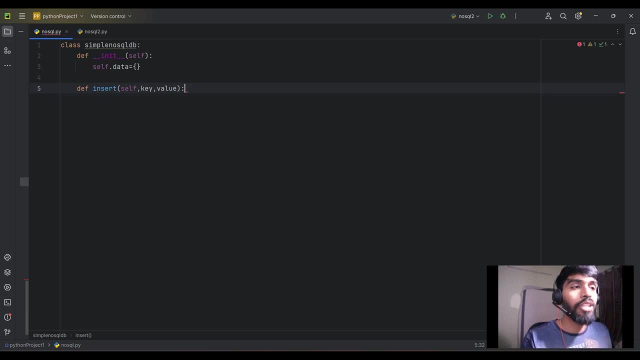 parameters to particular insert method, whereas key and value is what is our thing to insert. okay, as a parameter for This particular method, insert, fine. So now what I'm going to do is I'm just going to write a loop. if key the key, whatever I'm passing in selfdata. So selfdata is actually. 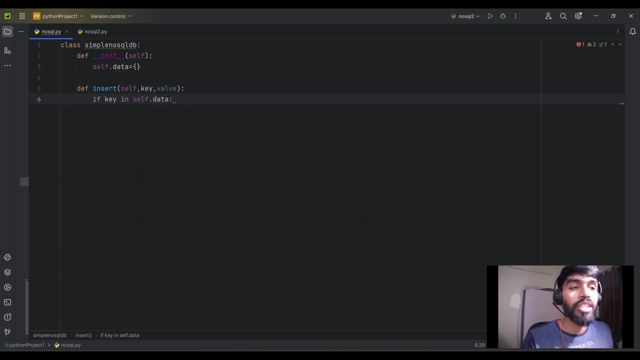 a dictionary. right Now it is empty. but I'm just checking whether the key, whatever they have given, is present inside the data. Okay, so if it is present, then I'm just printing it, print f And then I'm just passing the actual key. So key is this. first key is actually a string. 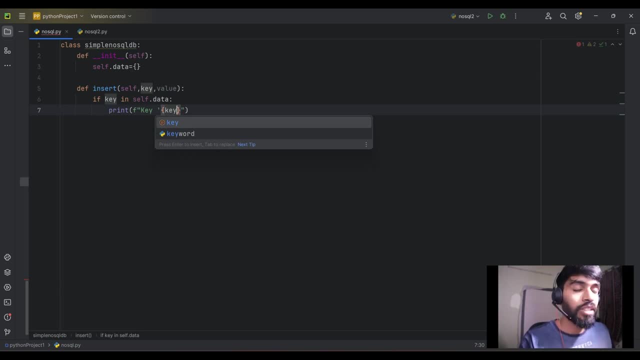 So the second key is a variable that I passed to my parameter. So the second key is a variable which I'm passing as a parameter and I'm referring it, So I'll just do already exist. So here, if key present, it says it is already exist and I'm just updating it. So if you take HBase, 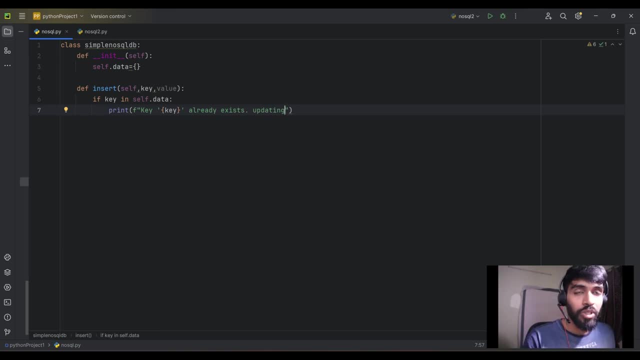 right, HBase accepts only unique row keys. Okay, row key means in HBase it's called as a primary key. So if you are inserting some key, it doesn't it will do. HBase will do an upsert. 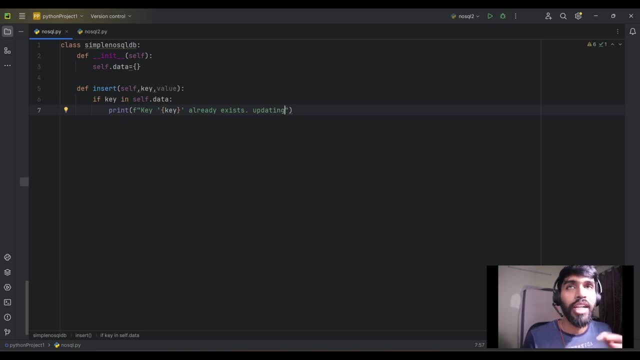 If the key is not present, it will insert. If it is present, it will update. So that is what we call it as an upsert. So now I'm doing that. So if the value is already there for the key, it does the update, else it do the insert. So print statement. So this is: 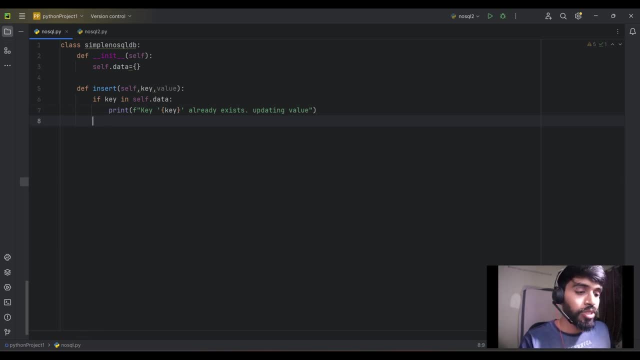 just a print statement. So now the action is: I'm just doing selfdata of key, Okay, Equal to value. I'm just doing the insert here. So now print, I'm just saying like inserted key and then the respective value. 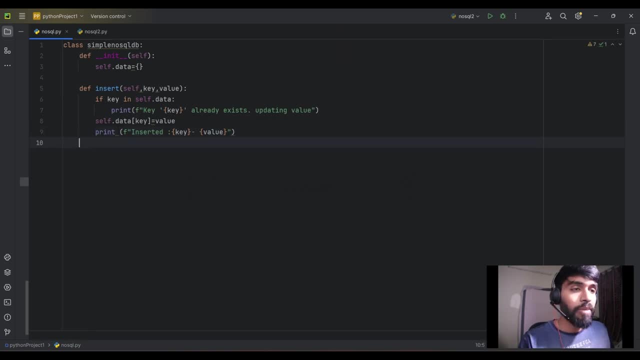 Okay, So now I'm done with the insert method. So now next thing, what I'm going to do is: so here the magic happens with the line number eight. Okay, So either it could be an append or update, or it could be an insert, Like we call it as an insert. sorry, upsert, We. 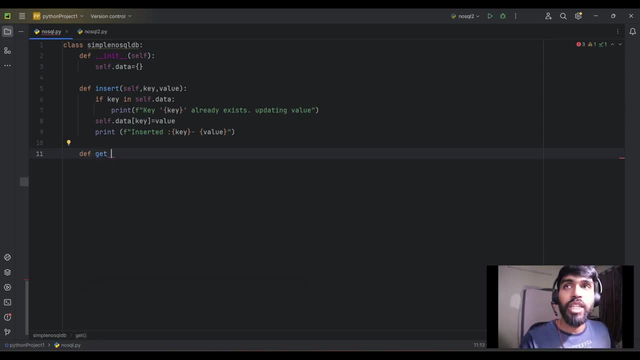 call it as an upsert. So the next method: now I'm just going to create get. So in the get what I'm going to pass is just the key and the respective. the whole record should come. That's it. Return: selfdataget of key. That's it, Simple, It's all done So now, whenever I invoke the 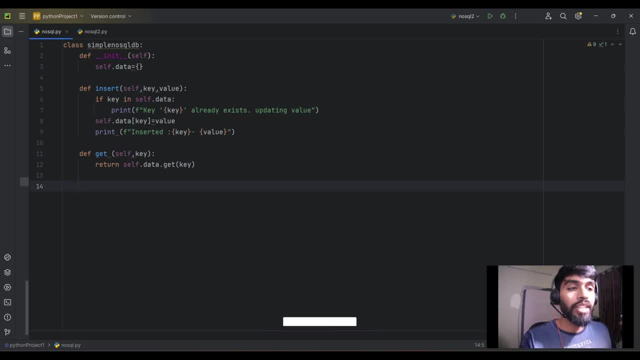 get method. I pass the key there and then I'll be getting the values with respect to the key with the line number 12.. Okay, So now I have to do delete, So I'll just create a method as delete And then selfdataget of key. Okay, So now I have to do delete, So I'll just create a. 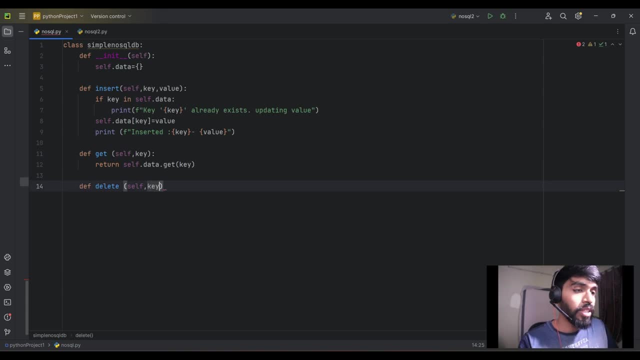 self of self comma key. So here key is an input for this delete method. So now, if key in selfdata, right, So now I use the function del. So del actually deletes the particular data from the dictionary based on the key. what we have given, That's key, Right So 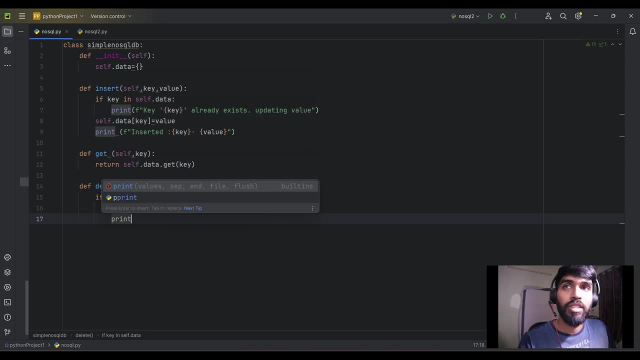 key. so now i'm just do the print statement. i'll say like deleted and then key. so i'll just print the key which is got deleted. okay, so now if the record is not present, right, so then i have to write the else condition, right? so i'll just do a print and i'll say like f key. 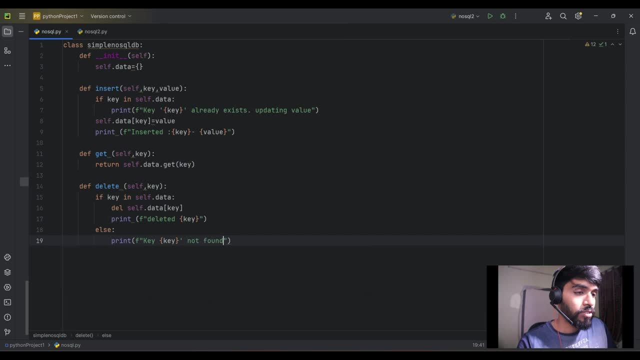 dot com. that's it right. so now the delete functionality is also completed. now the last thing is display, like output that i have to show when they do a select right. so uh, in hbase we have a command like scan which will display all the records. so similar to that i have to. 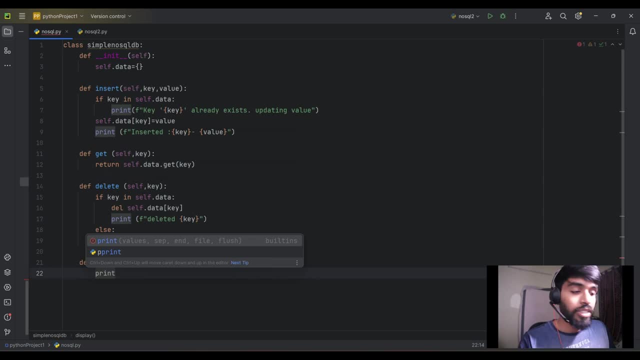 create a functionality here. so print: i'll say: like all e value. so i'll say like all e value. okay, so now i'll just write a for each loop, for each key comma value in self dot data, which is the dictionary. so i'll just call the items function. 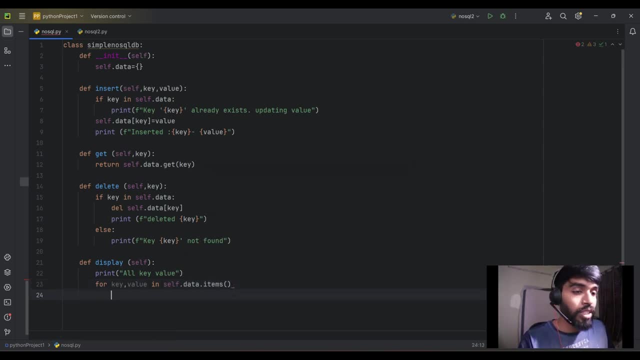 so it just iterate the dictionary and it will print all the key and value pairs. so print e and then your value. okay, so now, like okay, so now the display function is also done. so now we have to invoke this, right. so now what i'll go, what i'm going to do? i'll just create an object for the class and i'll be. 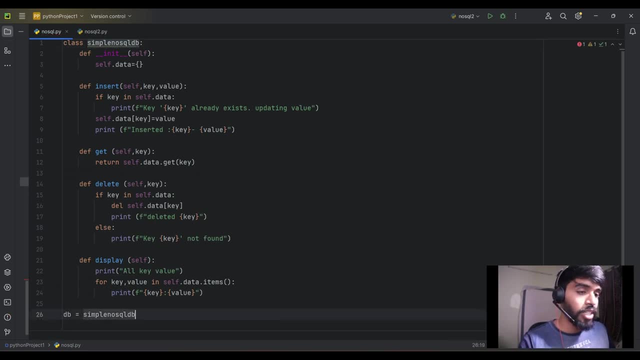 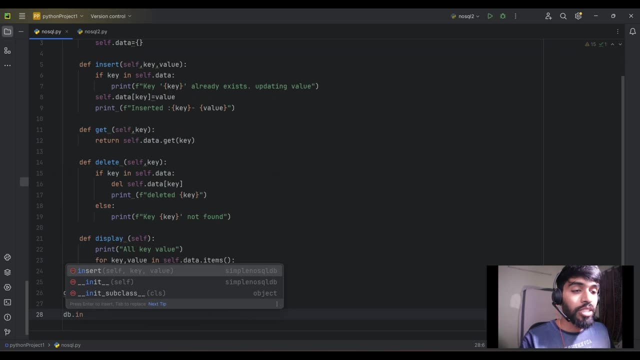 invoking it. so simple. no, sql, db. i'm just creating kind of an instance, uh, and then so with this what i'll do? db dot, i'll just do the, i'll just invoke the insert function and then i'll insert some values. now, so zero, zero one is a key i'm giving for the first row which i am going to insert. 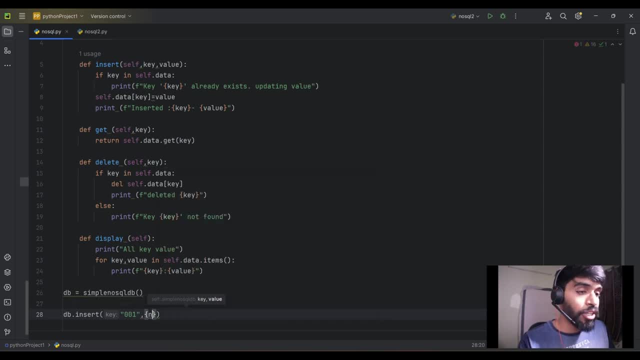 and the values is going to be in the form of key value pair- it's a dictionary, actually. so name and then colon. i'll just give gautam, and then this is one column. okay, this is one column, and the next column is going to be an age, and i'll give 30 and then comma. so the next is: 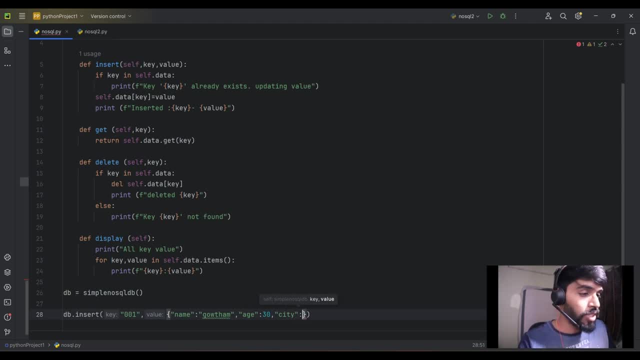 going to be city, i'll be giving chennai. and then the next one is going to be salary. okay, so i'm not going to insert salary now, so i'm just giving, uh, three key value pairs. just imagine: name is a column, age is a column, city is a column and gautam is a value, 30 is a value and chennai is a value okay. 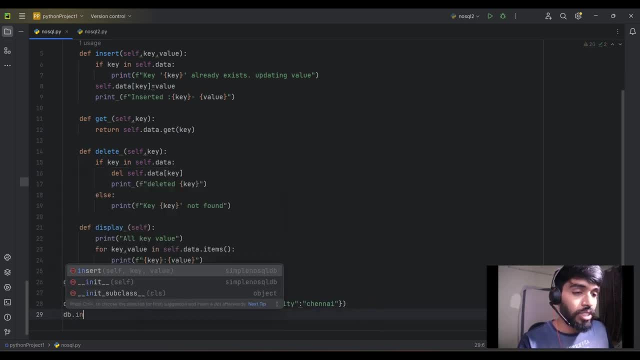 so now what i'm going to do, i'll just do one more insert insert. okay, i'll just copy and paste the above line. okay, so i'm just doing an another insert. so here i'll just change the name, i'll just put nandu, and the age is 28 and the city is going to be. 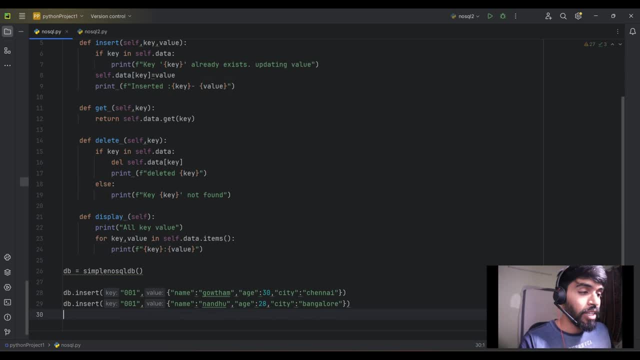 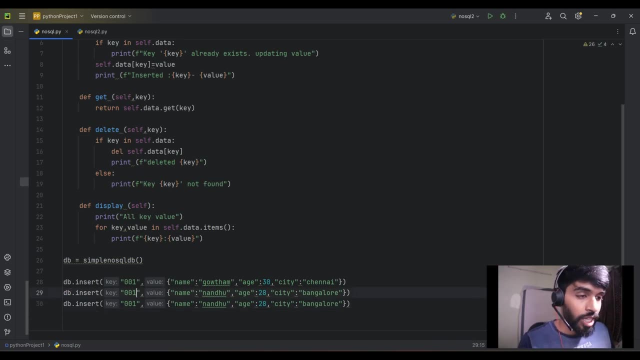 bangalore. okay, fine, so now i'll do another. uh, like, i'll just copy this again and i'll paste it here. okay, so here i'll change. okay, i'll change this. for second row, the key is going to be 2 and for the third row the key is going to be 3. now name is going to be saro and then age is going to be 31. 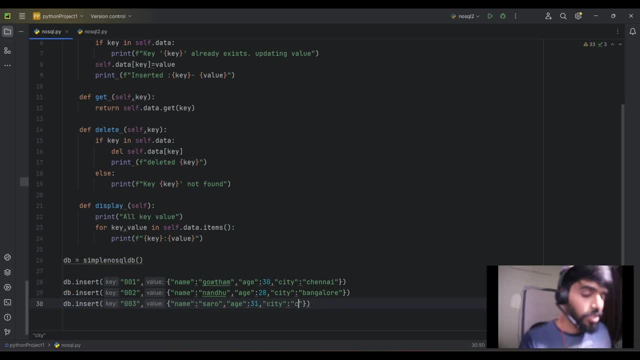 and city, i'll just put and city, i'll just put chennai again. and here i'm going to add one more column as a salary. okay, so you can ask me, like, how this is possible. see, in no sequence i'm going to use the space🤬 to insert my salary on, let's say, let's say, 10 coins a burqa. 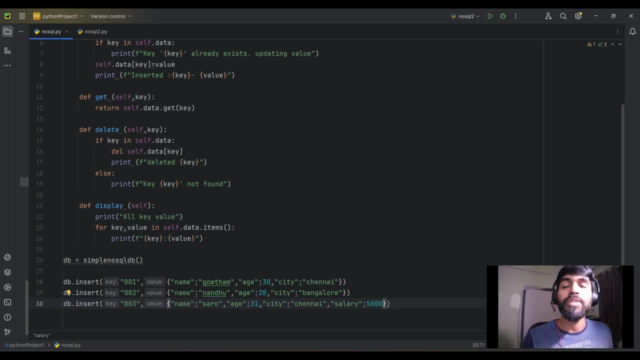 SQL, especially HBase, can have one record can have three columns, and second record can have four columns and third record can have five columns or even one column. So this is a schema less DB, right? No, SQL database means it's a schema less. So that is what an example I wanted. 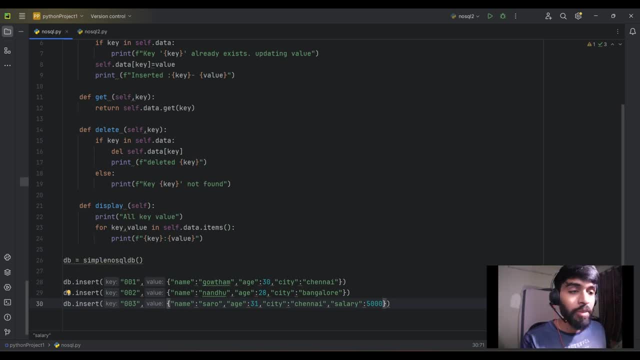 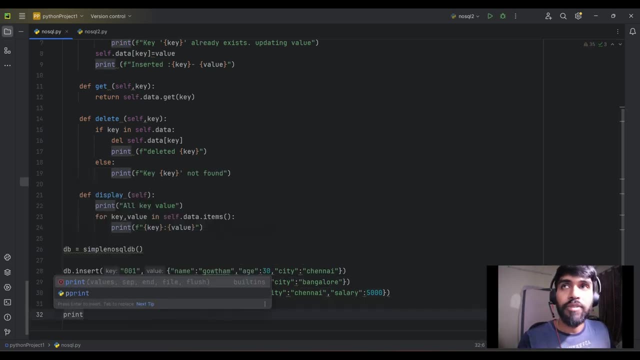 to show you here. Whereas the first two records has the same amount of column, but the third record has a different column. It is completely acceptable, right? So now what I'm going to do, print: I'm just give, get. okay, I'll just skip. get the first record, 001.. So this is a part of 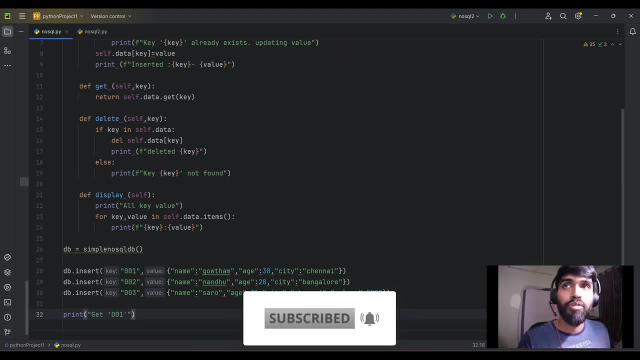 print statement: Okay, So this is going to be a part of print statement only. Okay, comma. So now DB dot get. so you have to pass the key. So my key is going to be 001.. So this is my key. So now I. 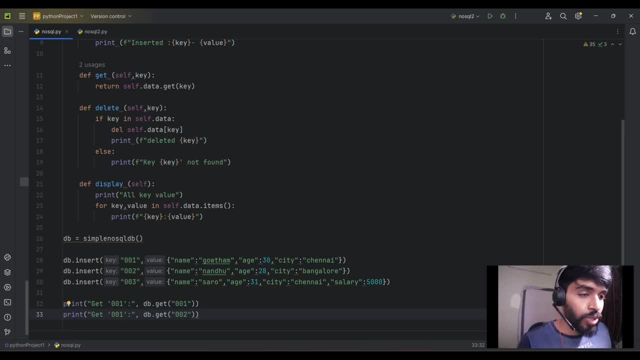 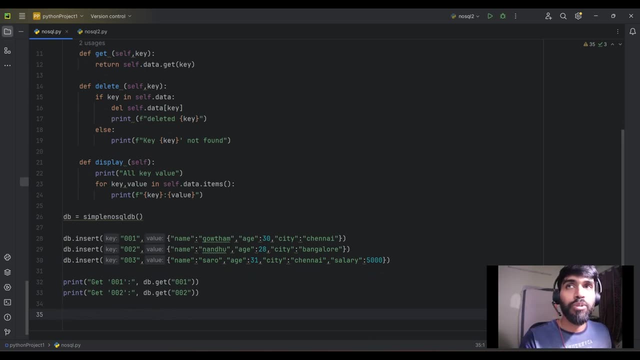 want to print my second record, So let me change it to two. And here part of print statement also I'll change it. So now what I'm going to do is so here I'm just showing you the print part. Now what I'm. 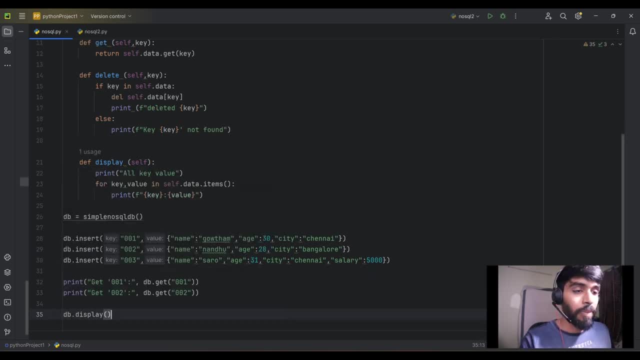 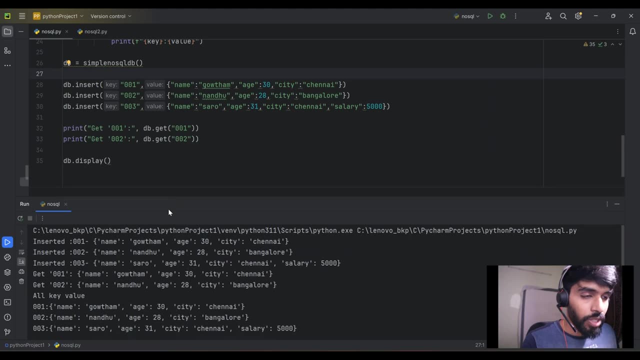 going to do DB dot display. So now let me run this code. Okay, you can able to see here. Okay, it says 001 is inserted, two is inserted, three is inserted: Okay, so, because inside insert I have a print statement. 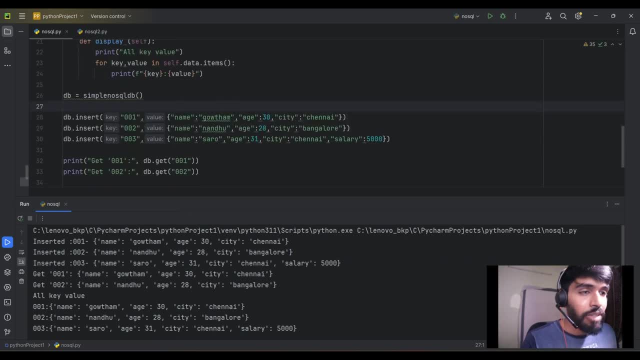 it is getting displayed. Okay, what is the next thing is I'm just printing these two, 001 and 002.. That you can see here, with the get as a print statement, as a string, you can able to see these two. I'm. 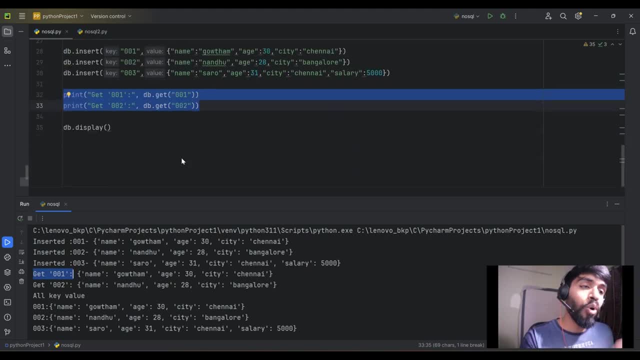 just I'm just printing it. Okay, now I have to print all the values and keys- key values- from the table. It's like select star from the RDBMS right And in HBase we call it as a scan table name. So here you can see all the record has been printed. So that is the display Now I have. 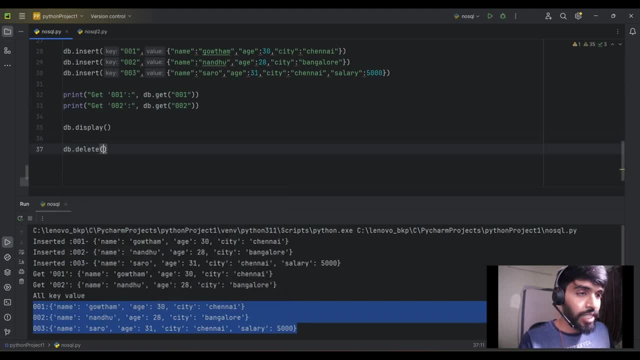 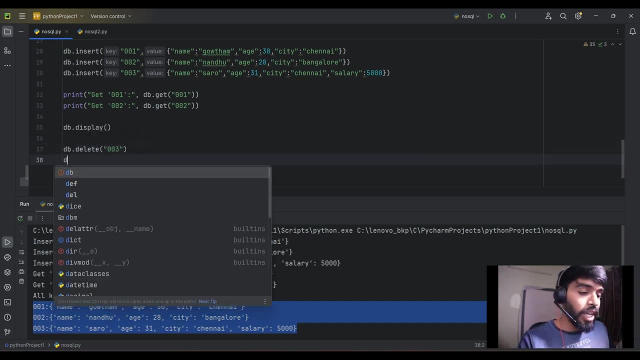 delete function also right. So let me do DB dot delete. and you have to pass a key, So let me pass 003.. So 003 has to be get deleted. So again, I will invoke DB dot display. Now, if I run this code, 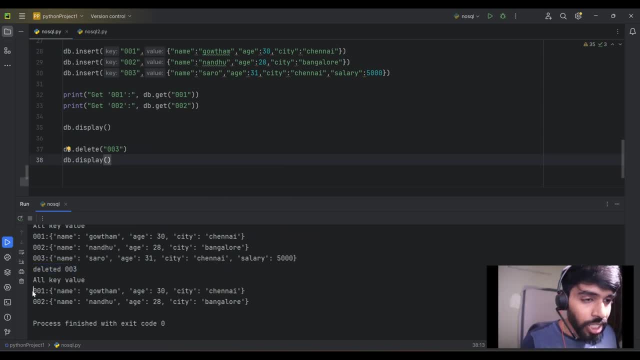 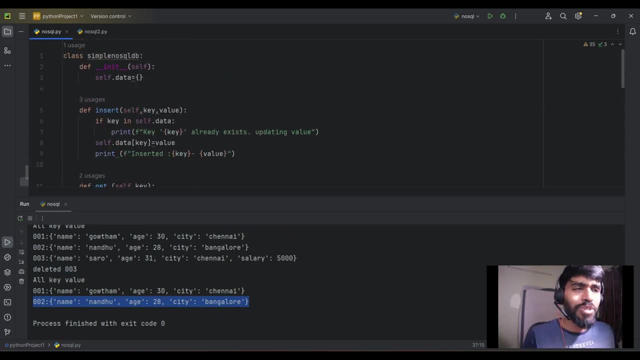 you can see, see deleted 003 and you're getting 001 record and 002 record. only Now you can ask me here. So the thing is like it's a very- seems to be a very- static code. right, You are just playing. 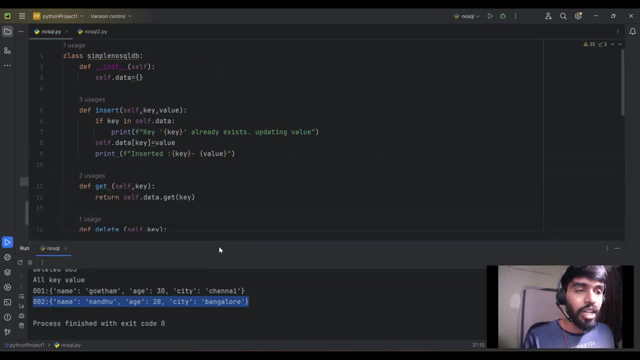 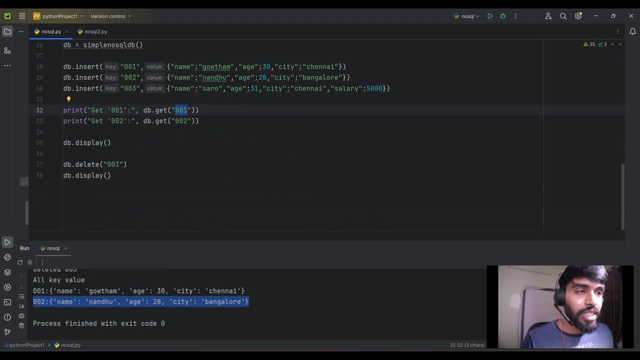 with the dictionary. Now we have a few functionalities, right? So what about? I have to select only one column, right? So here you cannot do that. If I give 001, it prints the complete row with all the columns. So now my thing is: I have to print only the name column, or I have to print only age column, So that 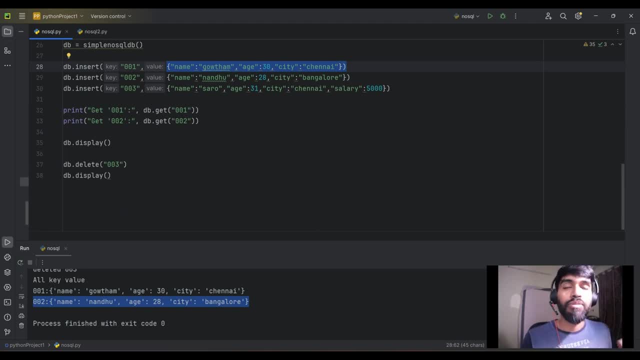 case was not satisfied by this code. And the second thing is: what about if I write a var condition right, So for example age equal to 31, only those record has to be get retrieved. So that is also not been satisfied. 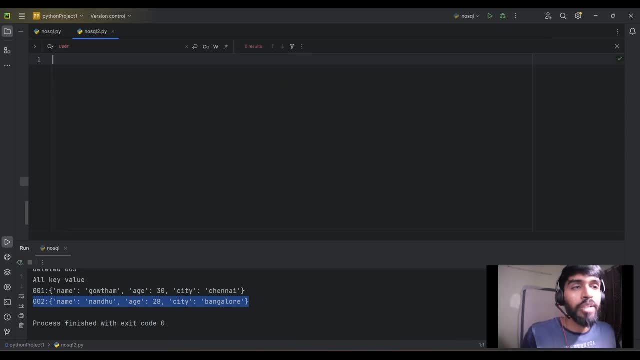 Here. So that is where I have written a second code. So so let me write a second code for this. So now I'm going to create a parent dictionary which is empty. So now, how I'm going to handle the situation of implementing the var condition, also selecting a particular column right. So I'm going 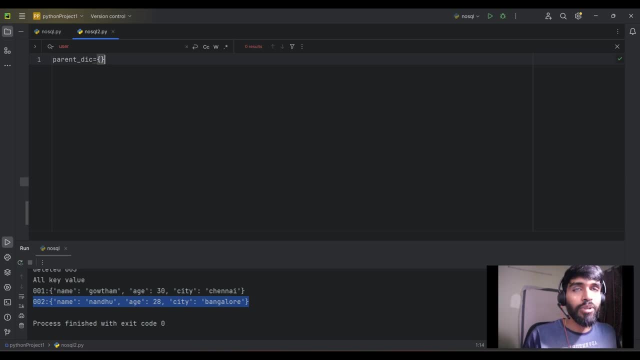 to create a parent and child dictionary. So child dictionary. so each and every, for each and every record, I'll be creating one child dictionary And these child dictionaries will be part of a parent dictionary. That is what this parent underscore dictionary. So one parent dictionary will have multiple child dictionaries And that means each. 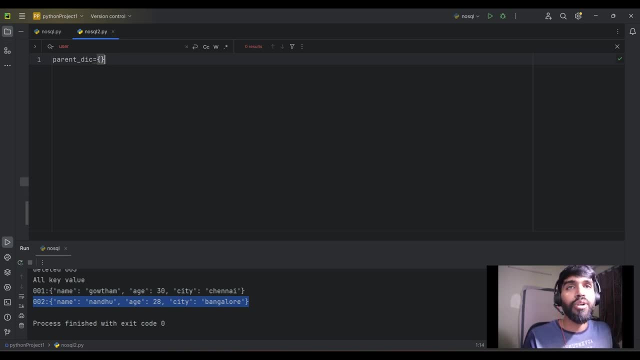 of the child dictionary is a record In the previous code, for I created one dictionary And within that dictionary I added so many records right, So now it is not like that actually. So now I created a parent dictionary, So now what I'm going to do is so I'll be creating two dictionaries. 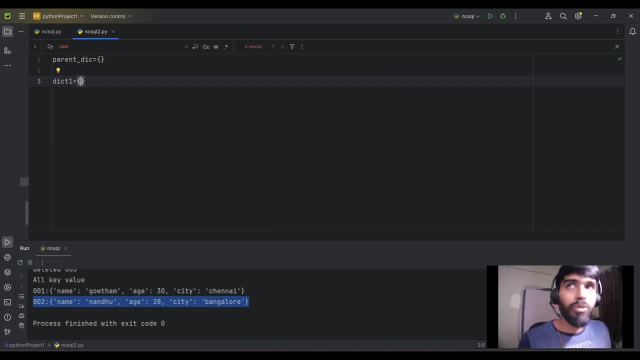 now dict one. Okay, so within this, what I'm going to do, I'll bring back the same record from here. Okay, I'll just. I'll just copy this. Okay, I'll be. I'll be loading within this, Okay, So now again the same thing. 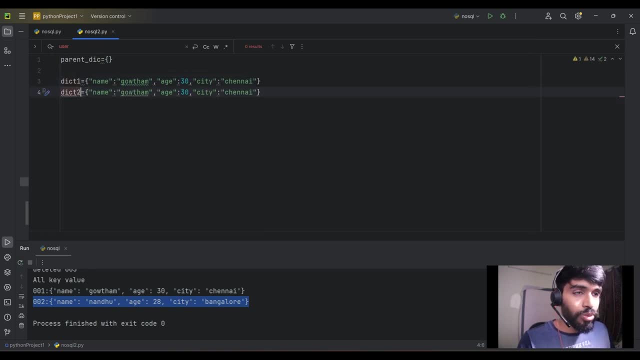 I'm going to do, but I'm going to give a name as dictionary two, dictionary two, And instead of name I'll change this to Nandu, And age is going to be 28.. Let the city be the same. So I have two. 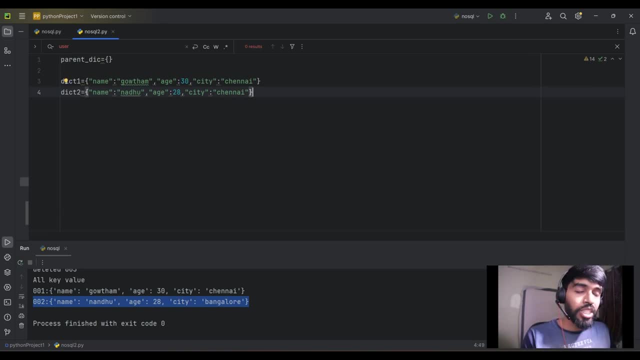 dictionaries here. So before I created within for one dictionary, I created so many records, but for each and every record I'm creating a separate dictionary. Okay, So here also, let's build this as a schema less. So let me add one more additional column to a 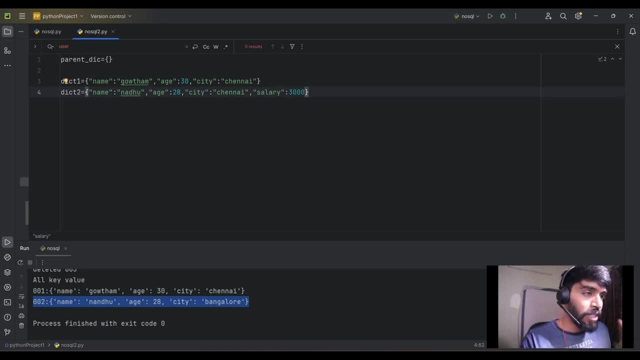 different record. I'll just put 33,000 here. So now I created two dictionaries for each record, one dictionary, Fine, So now what I'm going to do. so I'll assign these two dictionaries dict one, and dict two is actually the child dictionaries. okay, to my parent dictionary. 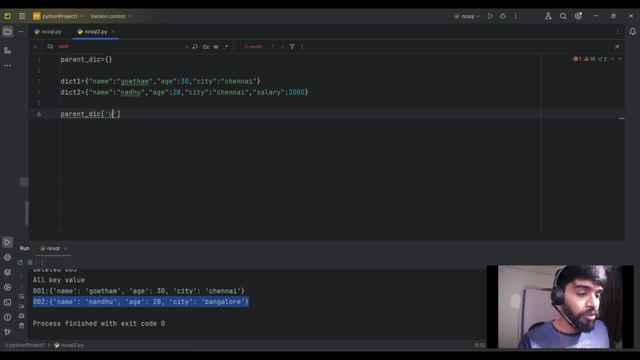 So parent underscore dictionary, I'm giving a name for it, So user one, one equal to dict one. So the same thing I'll be doing for the second, So dict two, and then, and I'm going to store this as a user two in my parent dictionary. So now, parent dictionary is: 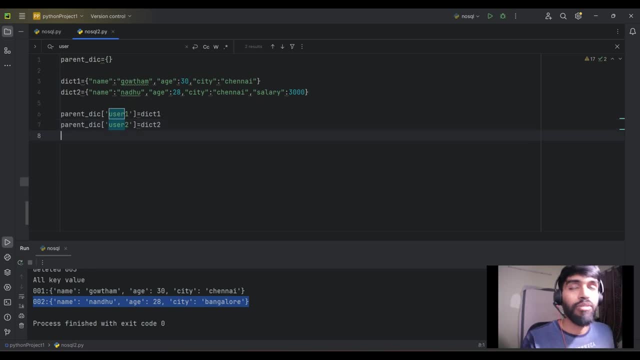 same, but it has two child dictionaries. Fine, So now I'm going to print, So I'm going to print comma. Okay, so before printing this, what I'll be doing is: so I'll just give a name for this: parent dictionary of user one and then parent dictionary of user two. I'll just give a name for. 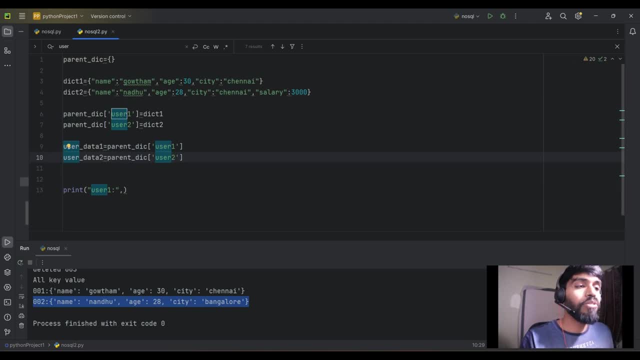 it. Okay, then only I can use it in the throughout my code. I can use this as a variable name, right? So yeah? so now what I'll be doing is I'll just print this user data one. And now what I'm going to do is, for the second record, I'll be doing two. okay, two dot. 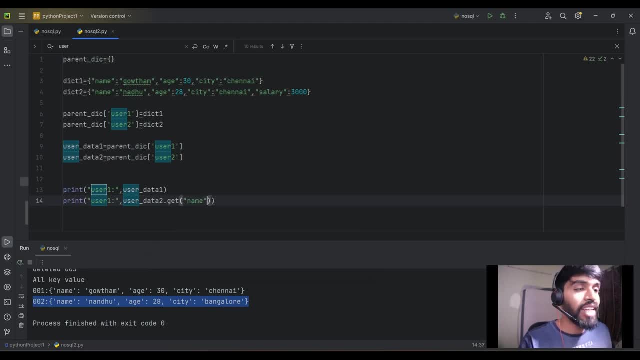 there is a function get, And within this I'll be printing name. So that means you are selecting only the name column instead of selecting the entire row. So line number 13 will print the entire row. line number 14 will print only the second row name column. it's like select name. 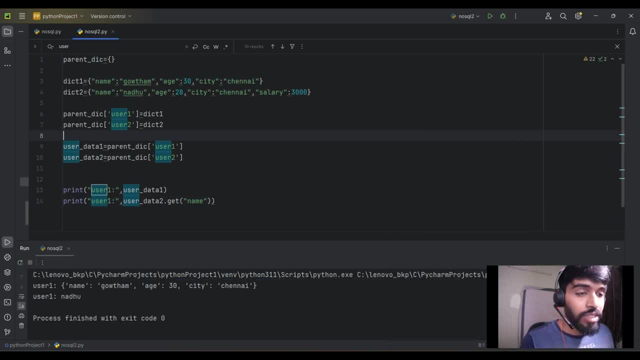 from the table. Now let me run this code. Okay, you can see user one. okay, so let me change the print statement here to user two. I'll rerun the code again. Sorry for that. Okay, so user one name: Gautam. so whole record with all three columns, but in user. 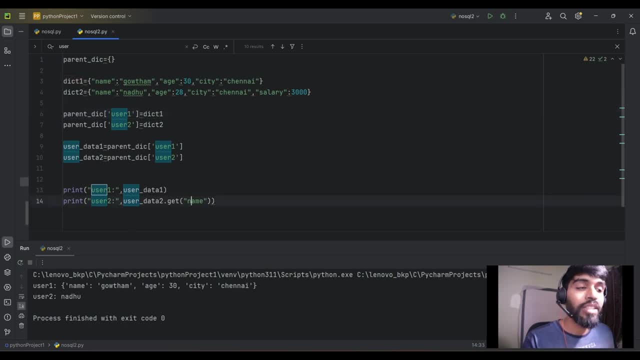 two, you can see Nandu as my output, because I selected only the name column. So it's like you comment this, you remove this and just put salary. Now again you run the code So you'll be getting 3000 as the output. right, So select part is done. So now what is the next thing that we have to do? 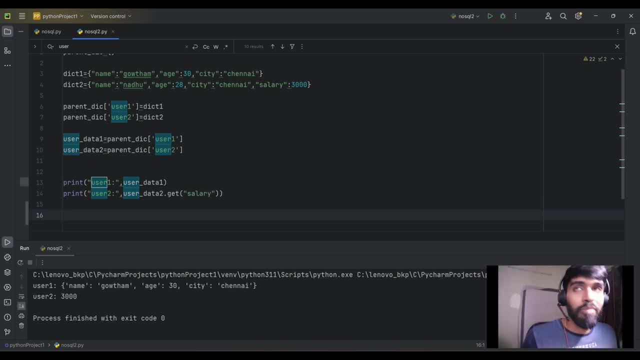 is, we have to work on the var condition. so i'm i'm just going give some conditions here and also, like you want to print all the records. scan all the records so that i have to again put a for each loop. so let me do that as well. key comma value in the parent dictionary. i'm just 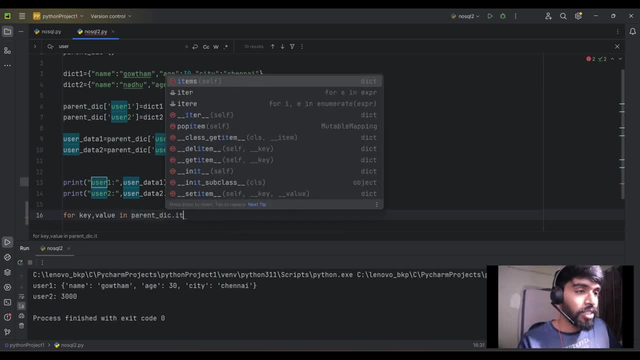 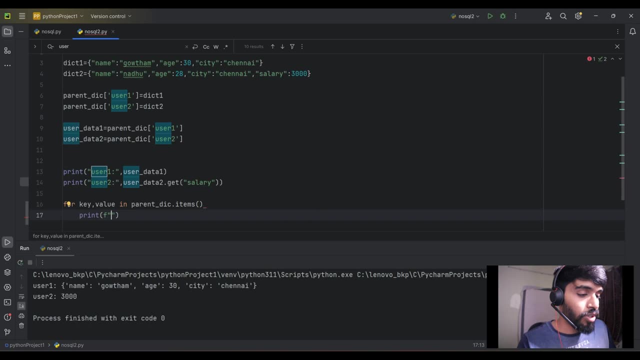 iterating the parent dictionary dot items. so inside this i'll be just printing f of e and then value. so this will print all the records okay. so just scan of all. okay. so this printed both the records all from the dictionary, whatever the parent dictionary has. parent dictionary has two child dictionary. 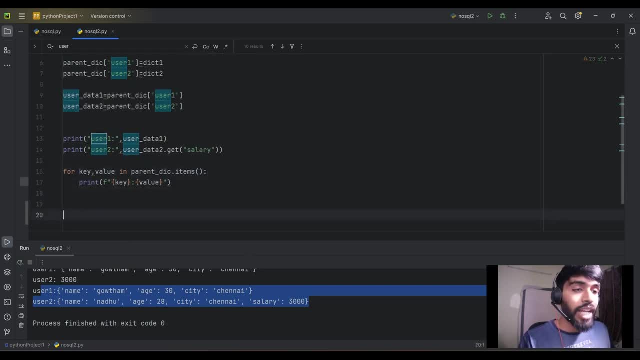 it just got printed. so now what is the next thing? so let me write a function here. so def find records. okay, so i'm just creating a method. so this method is for var condition. okay, so this find records. i'm going to pass three variable collection, comma, key, comma value. so that means: 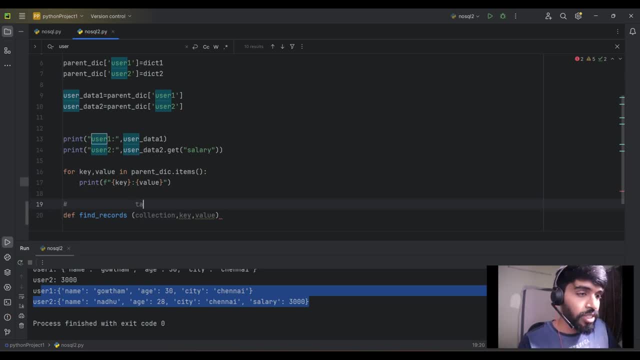 i'll just write a comment statement here. so this collection is like a table name and this key is like a column name, and then value is like a- the value, what you are giving. so it's like select. uh, so it's like select star from table name. 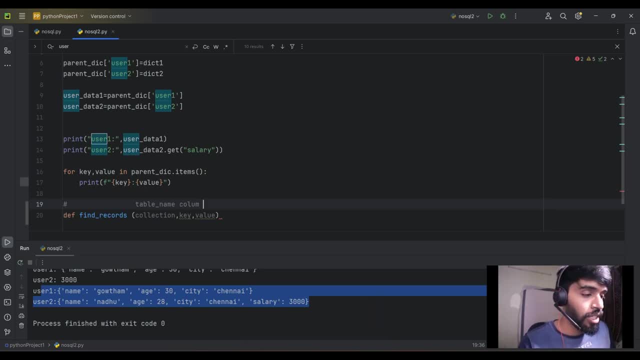 var column equal to value. so that is the equivalent query here. so equal to value. so i i just want to have three values to frame this query right. so i'm just getting the collection, which is nothing but your dictionary key, and then value. fine, so now what i'm going to do? i'm just going to create. 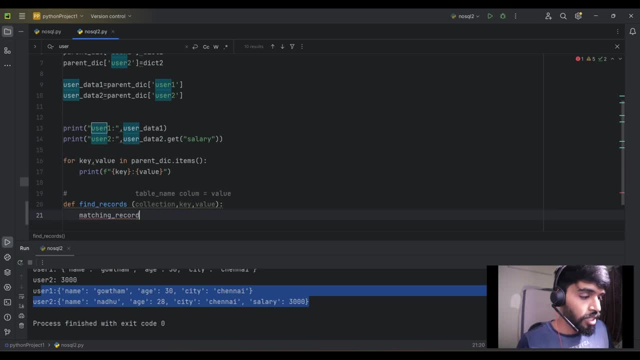 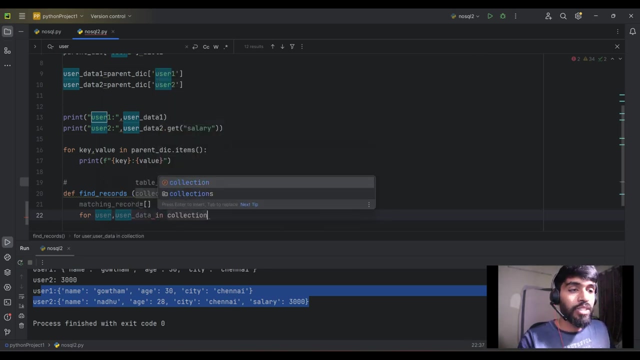 the empty, empty list called matching records. okay, so now i'm just going to write for user comma, user underscore, data in collection. so collection is the one which i'm passing dot items. okay, so it's like i'm iterating it. so before getting into the code, right, let me show you, like, how this method is going to. 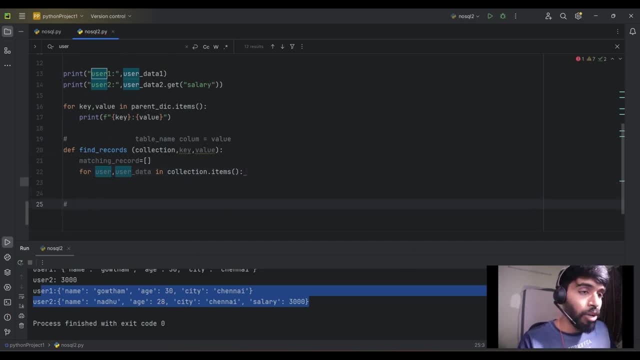 get called. okay, you will be getting an idea right. so now, how i'm going to invoke the method is find underscore records and the values, what i'm going to pass within this. right, so i'll be passing my- uh, this dictionary. okay, i'll be passing this dictionary and the key is going to be the age and value is going to be the 31, so 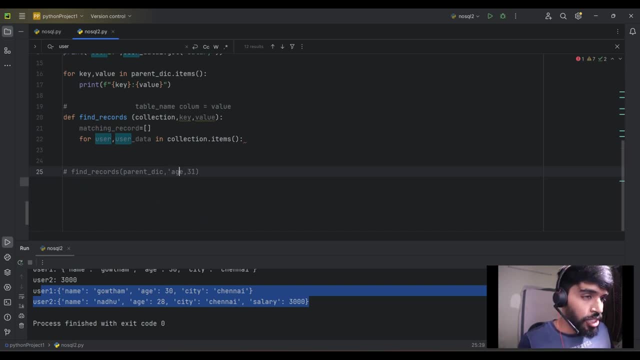 this is what i'm going to pass and that's mean: uh, the var condition is var select star from table name. var age equal to 31. so this is the input i'm giving for find record method. so now i'll be getting the record which matches with the value 31 for the age column. okay, from the dictionary. 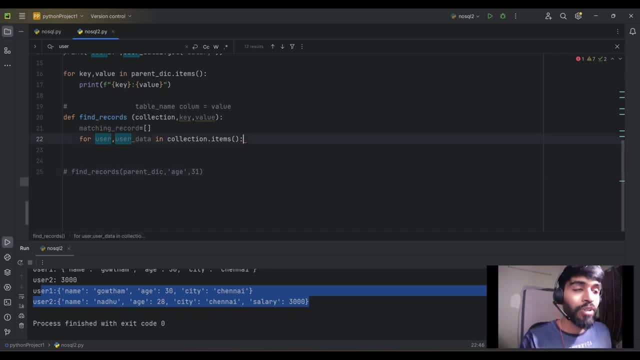 fine, so this is how i'm going to invoke this method. okay, let me continue writing my find record implementation. so i have- i'm doing a for each loop for the iteration to get all the uh values from the collection. so collection is nothing but your parent dictionary. i'm getting all i'm just 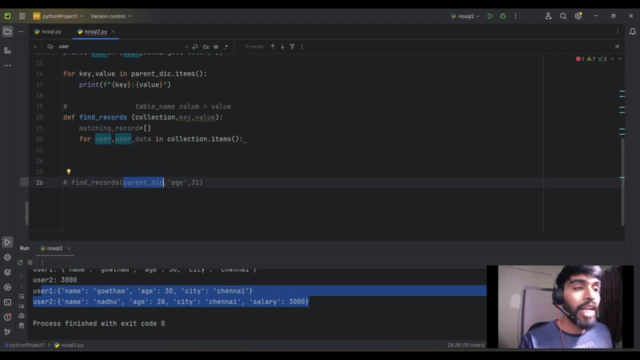 iterating all the dictionaries. the child dictionary is within my parent dictionary, so now i'm just writing an if loop. if key, whatever the key you are passing age is a key, so if key in. so if key and user underscore data of e, equal to e, equal to equal to value, then it has to enter into this. 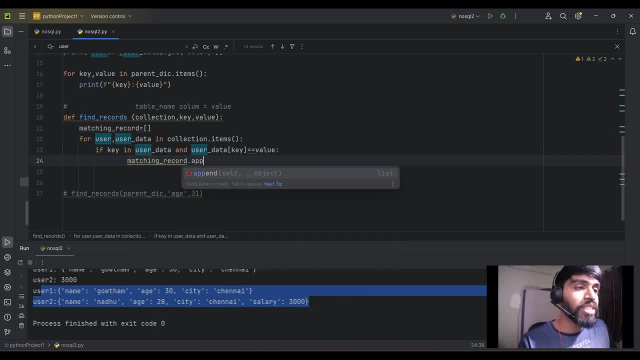 matching underscore record dot. i'm just appending it so i can have more than one records with the age matching age equal to 31, right. so if it is more than one record also i have to append it right. so that's why i'm just adding this append functionality. so user comma. user comma. user comma. 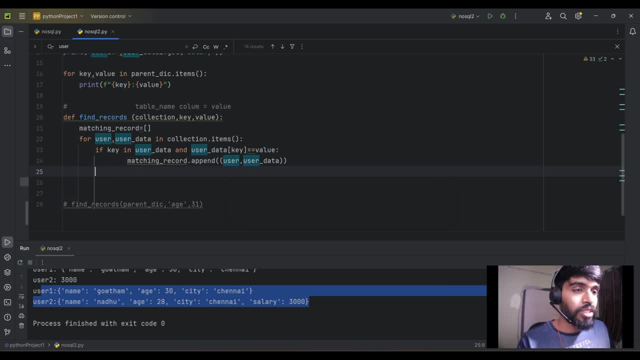 user underscore data and then i'm just going to return this matching record. that's it. so now i'm just going to invoke this. so what i'm going to do is match matching underscore record is my list, right? so matching underscore record is my list, so equal to find record of. i'm. 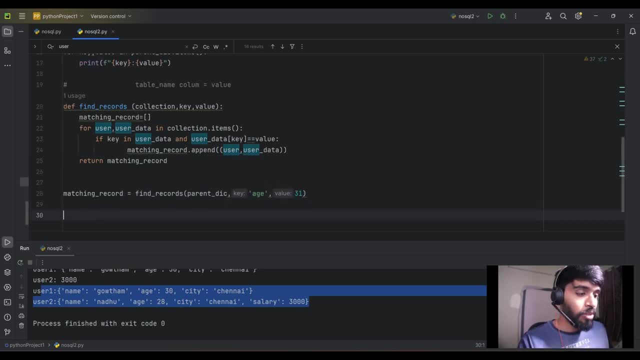 just passing whatever the values required to process. now what i'll be doing is i'm just iterating for user comma, user underscore data. so now i'm going to iterate this matching record because this is a list. so for user comma, user underscore data in the matching record, right? so 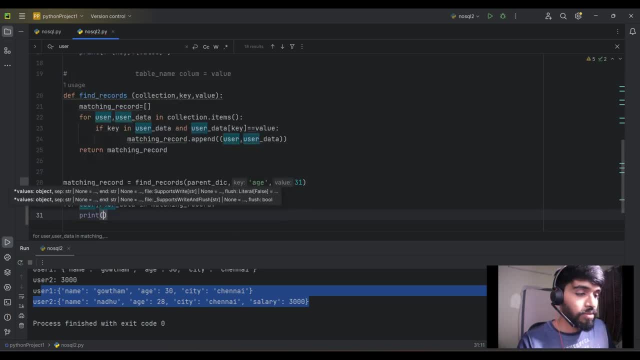 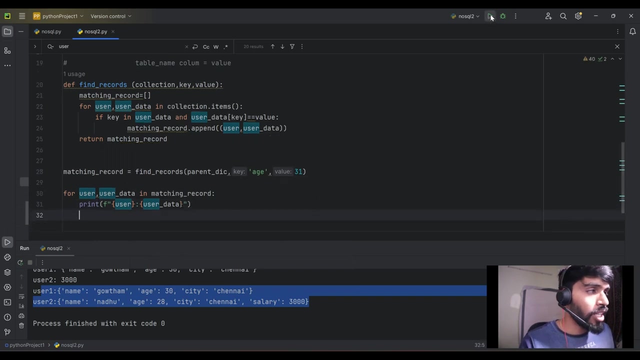 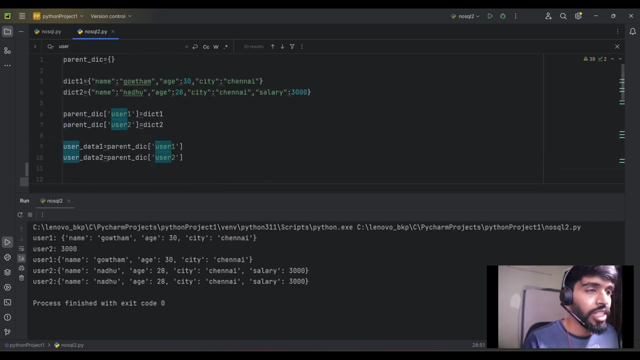 i'll be printing f of user and then user. okay, so now i'll run this code. so here i'll not get any record because i don't have 31 for the age, so i have ages 30 and 28. so let me change this to 28 and for for better readability. 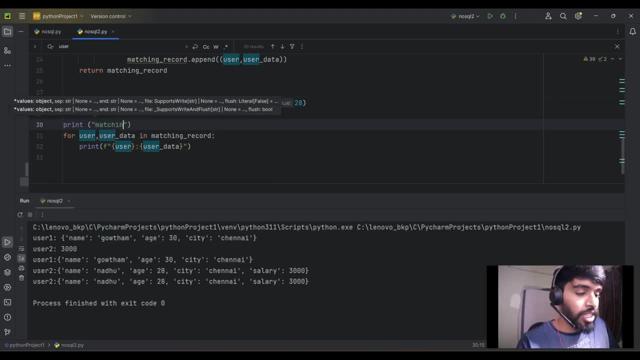 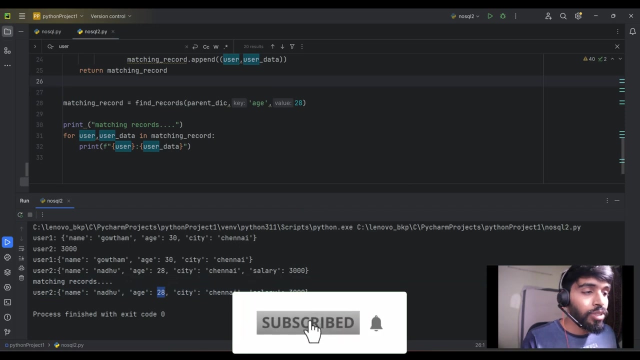 i'll be adding a print statement before the loop as matching records. okay, so now i'll run this code. okay, so now you can see under matching records, matching record, i'm getting only one record which matches with the age 28. so these two lines before this, you can see these two lines or the print statement that is coming from here. okay, don't. 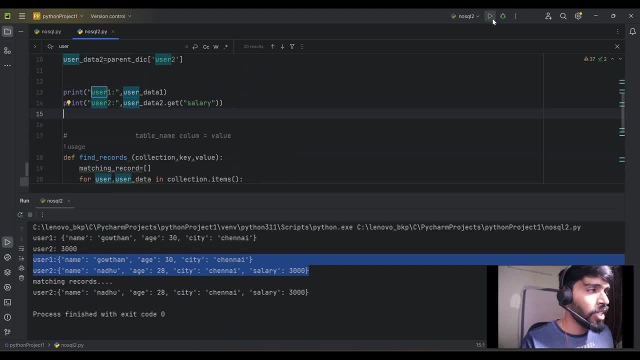 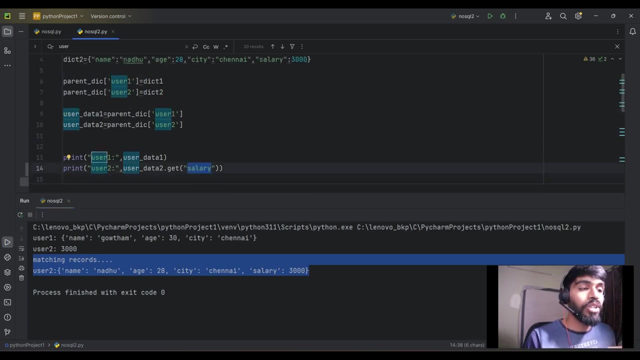 get confused, okay, or even i can remove this for each loop and i'll rerun the code, okay, yeah, you can see here. that is gone. that is gone, right. so now matching record is uh, 28. so there is only one record with the age 28- i'm getting it- and 3000 is something that select part. so now in this code i'm 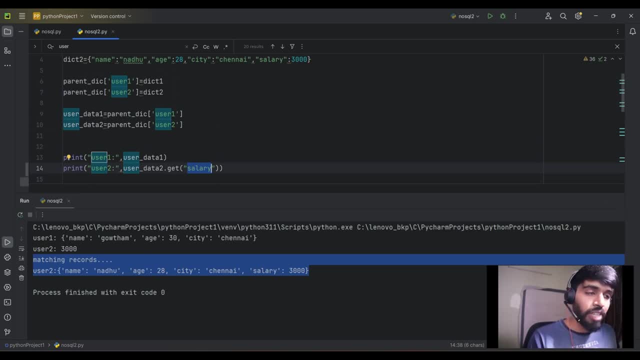 just going to print it and then i'll run this code over here. okay, and as you can see here in this code i'm just running the code. so i'll now run this code and it will pop up in my code and i'll be able to have it fill in the code with my values. so now i'm going to do the same thing. 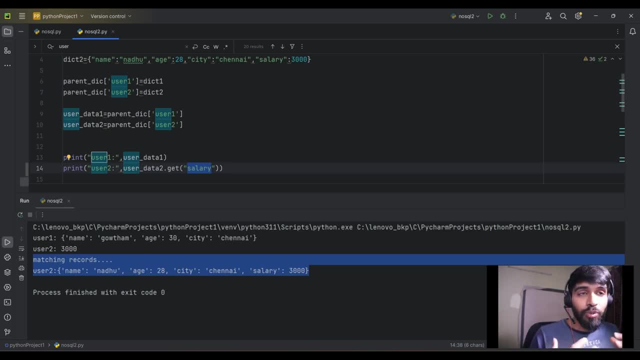 in this case, all i have to do is i'm going to be making a map right here and i'm going to be using the code to build this code, and then i'm going to start building the database to do the initial setup of this code. now, after this step, we are done with the first step, which is the. 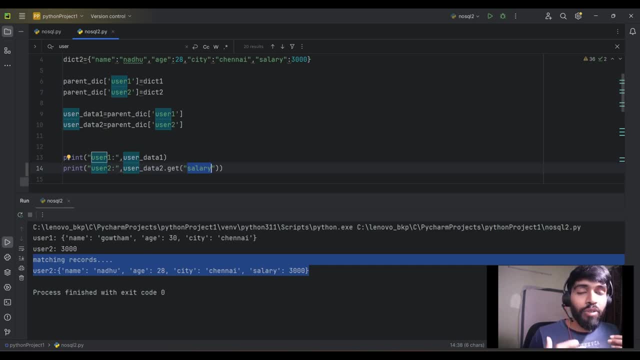 fast the algorithms for indexing, and then you have to add a lot of algorithms for supporting the storage formats and the output formats and the connector to connect with other technologies like spark or hive or cassandra. no sql to no sql database. so these and all as part of the things, 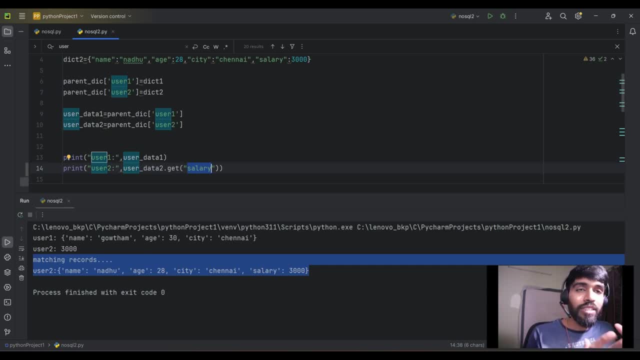 we have to do, but this is a outline, a structure. i'm proving that this is how a key value store, similar to hbase, how this works, right. so thanks for watching. if you really like this video, please do subscribe my channel for more such videos. and i have. i have given my instagram and linkedin in.